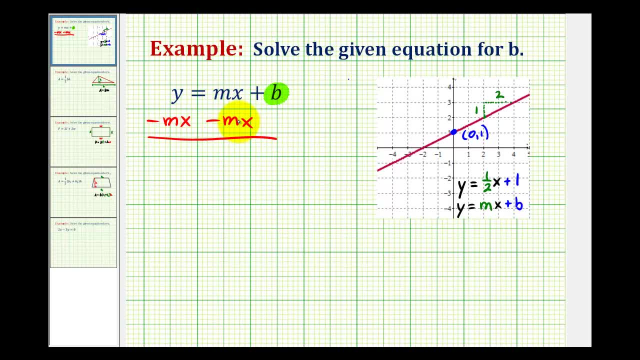 here we have mx minus mx, which would be equal to zero. On the left side we have y minus mx, and on the right side we're left with just b. So now this equation is solved for b. Let's take a look at the next equation. 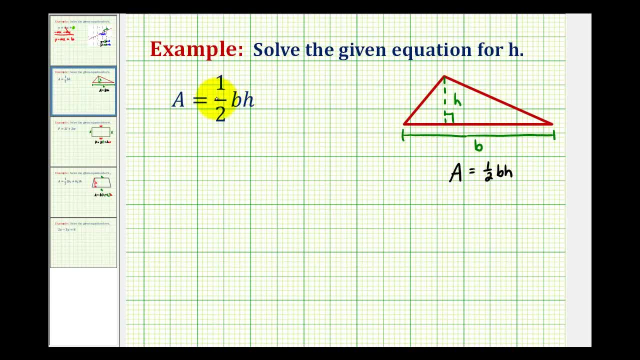 Let's look at another example. In this example we want to solve the equation: y equals one-half times b times h for the variable h, And this happens to be the area formula for a triangle, again as we see here on the right. So one-half b and h are attached by multiplication. 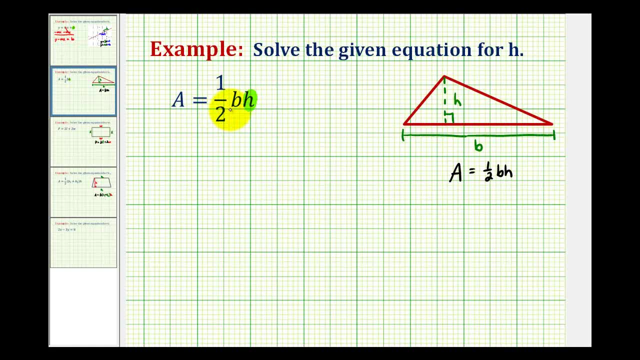 So normally to isolate h we would divide. but if we wanted to isolate bh first, instead of dividing by one-half we would multiply by the reciprocal. So in this case we'll multiply both sides of the equation. We'll divide both sides by two to isolate b and h. 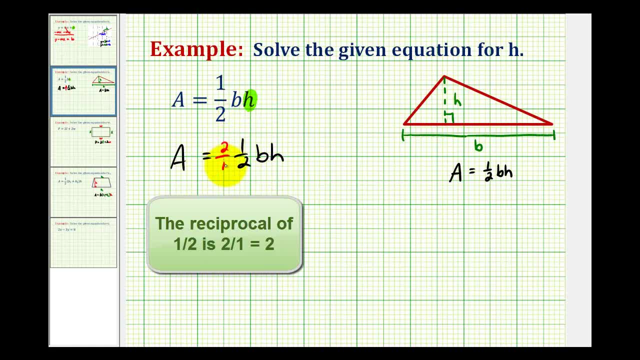 So on the right side, we'll multiply by two over one. On the left side, we'll go ahead and just write it as two, since this is in fraction form and this isn't So. now we have: two times a is equal to b times h. And now, if we want to isolate h, 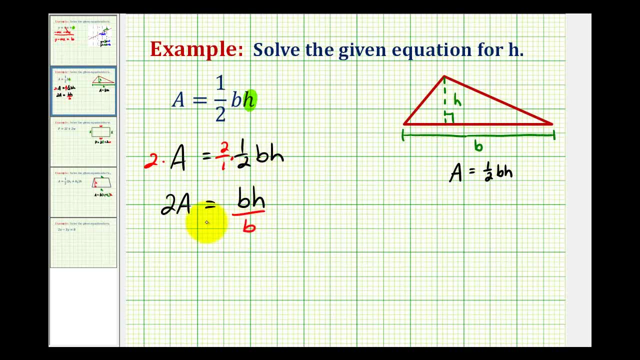 since this b is attached by multiplication, we'll divide both sides by b. So on the left side we have two times a divided by b is equal to h. On the right side, the b simplifies out and we're left with h. So now this equation is solved for. 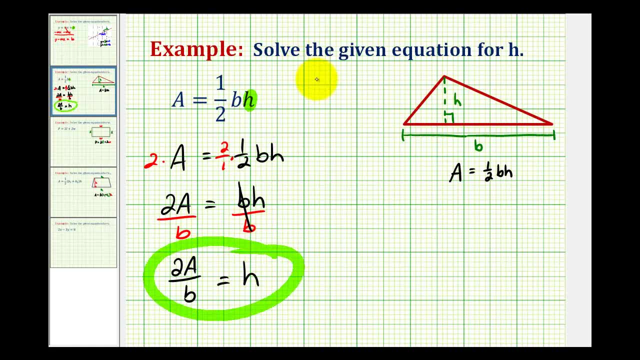 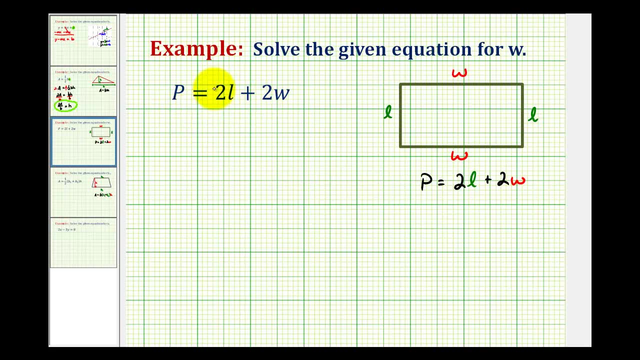 h. Let's take a look at one more example for this video. Here we're given the equation p equals two l plus two w, And we want to solve the equation for w, And this equation happens to be the perimeter formula for a rectangle. 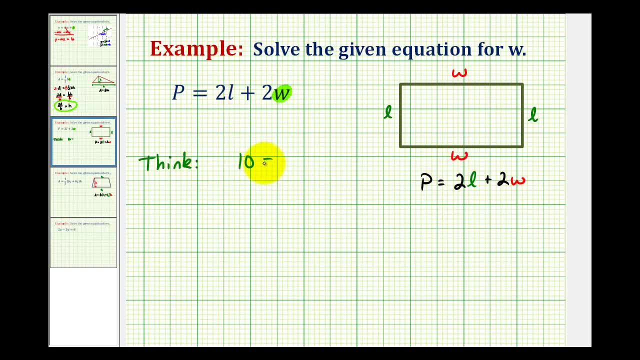 So again, if you can solve the equation- let's say ten equals four plus two x- You should also be able to isolate w in this equation. We know when solving this type of equation we would first subtract four on both sides And then divide by two.